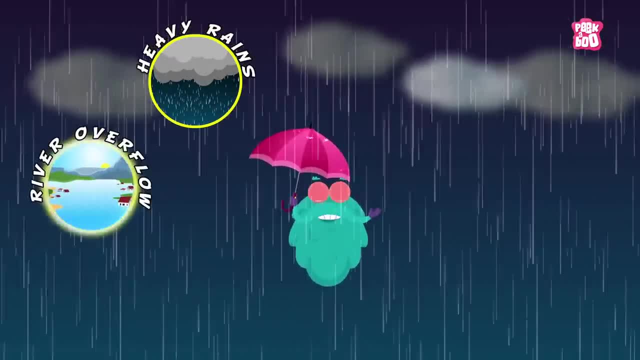 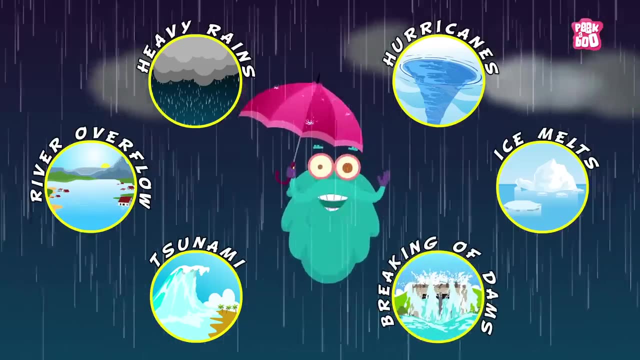 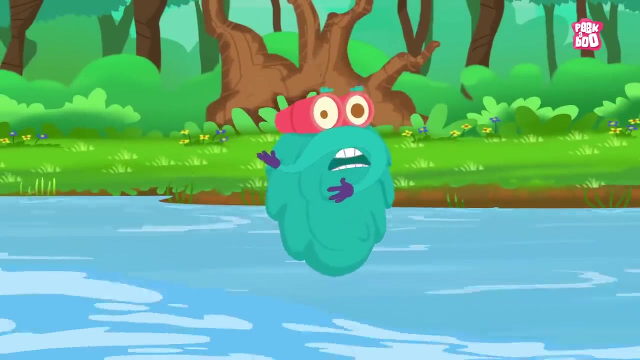 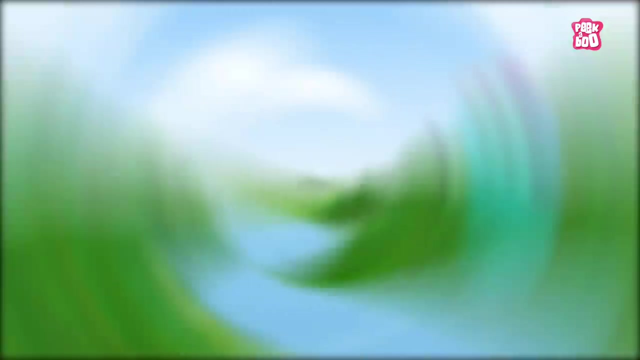 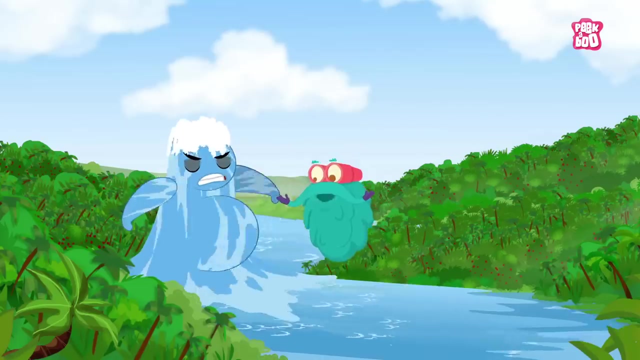 Causes of floods are heavy rains, river overflow, tsunami or hurricanes, ice or snowmills, breaking of dams, etc. Help. So a flood can be divided majorly into three categories: Slow-onset floods: This kind of flood usually happens when water bodies overflood their banks. 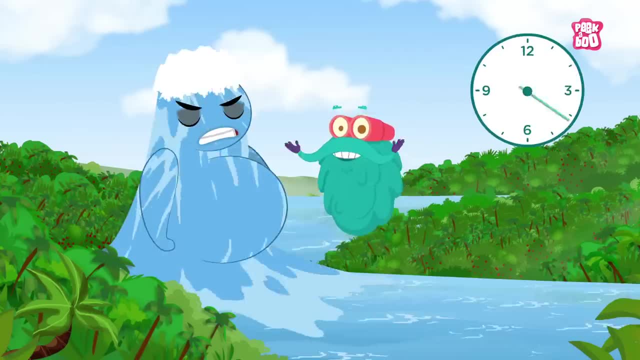 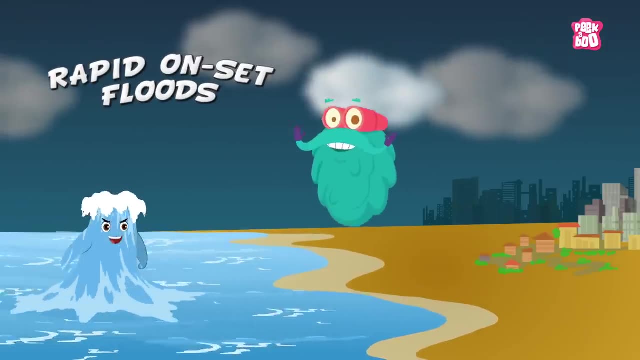 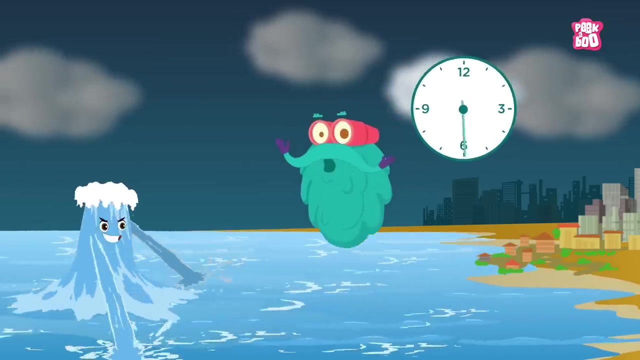 As the name suggests, this one develops slowly, which can last for days or even weeks. Rapid-onset floods: This kind of flood lasts for a day or two. Even though it is destructive, it still takes a little time to develop and thus giving people a chance to escape. 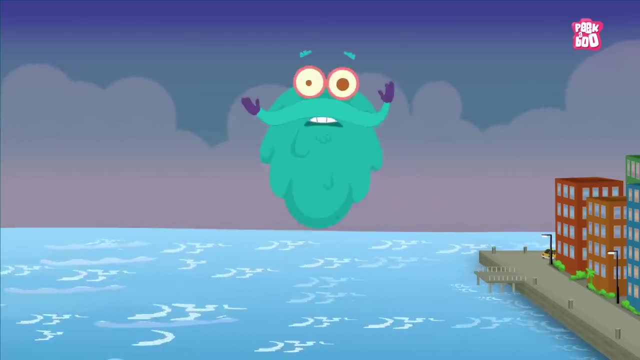 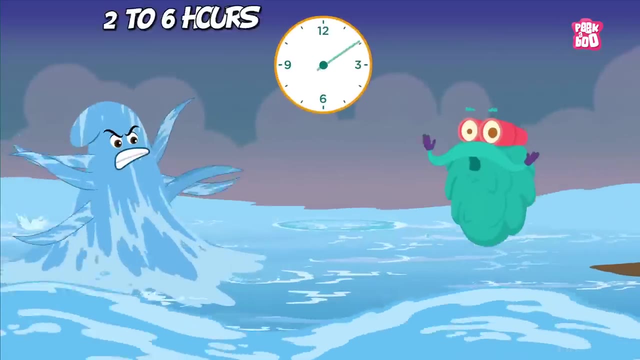 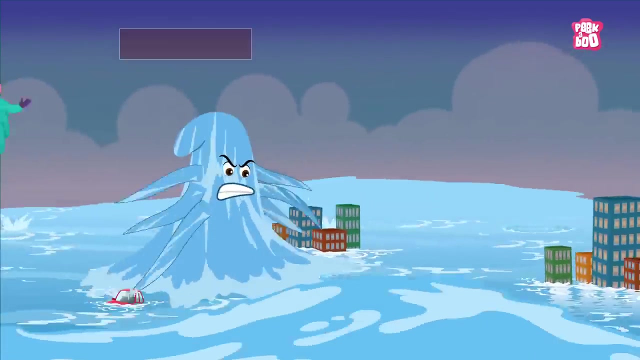 Now comes the most dangerous of them all: Flash floods. This kind occurs within a very short time, that is, 2 to 6 hours, and sometimes within minutes. This doesn't give any time to prepare. No warnings, no words of caution, just destruction. 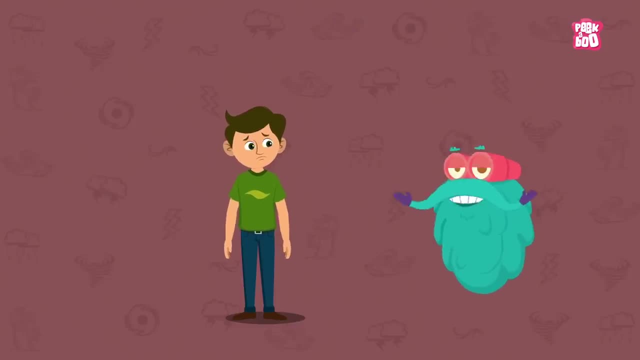 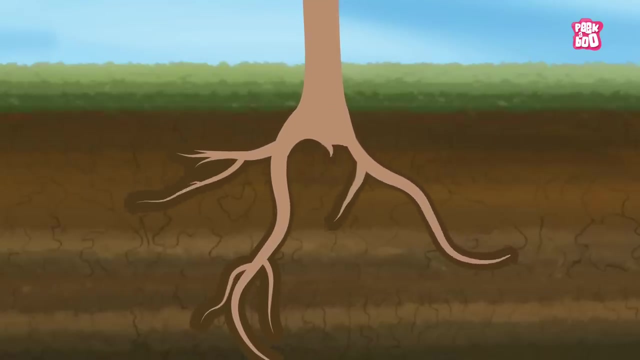 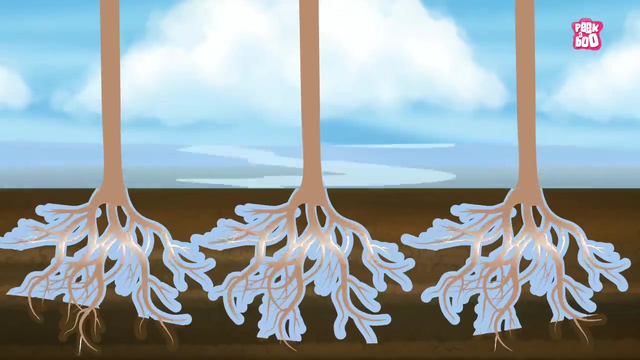 But hey, don't lose heart, We can do our bits to prevent floods. Yes, that's right. Planting more trees help preventing floods. The roots of plants and trees dig deep into the soil and create spaces between soil particles Which help in seeping and holding on to flood water. 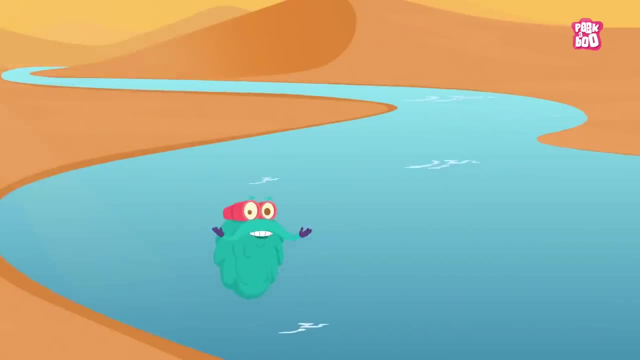 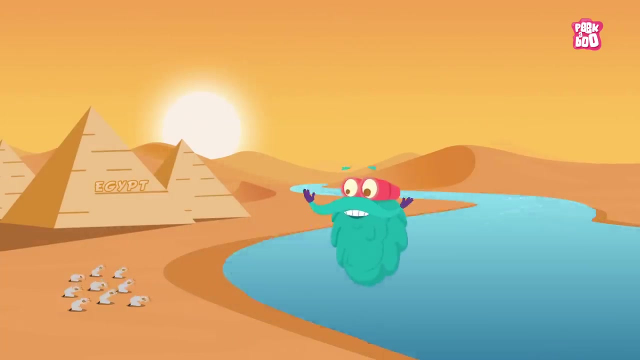 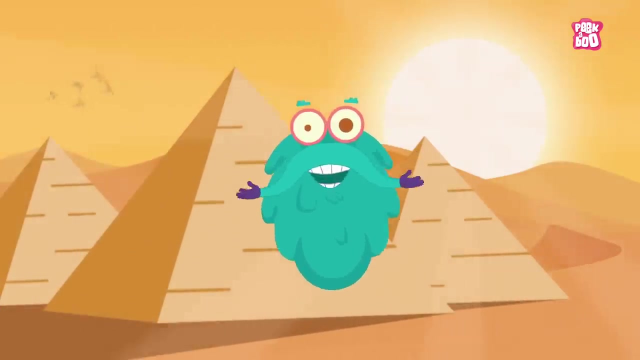 Trivia time. Floods can even occur in deserts. In ancient Egypt, people relied on the Nile River floods because they created enriched soil for farmers. So what are the three types of floods? Well, you keep thinking and post your answers in the comment section below. 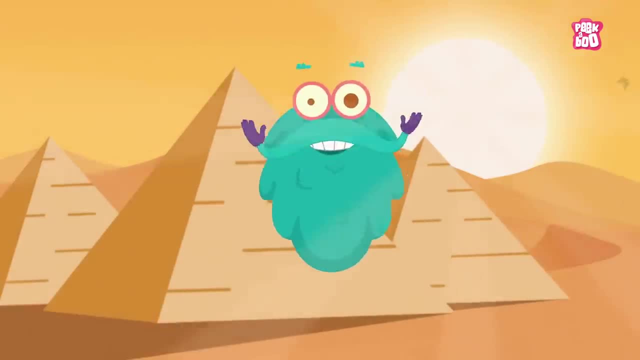 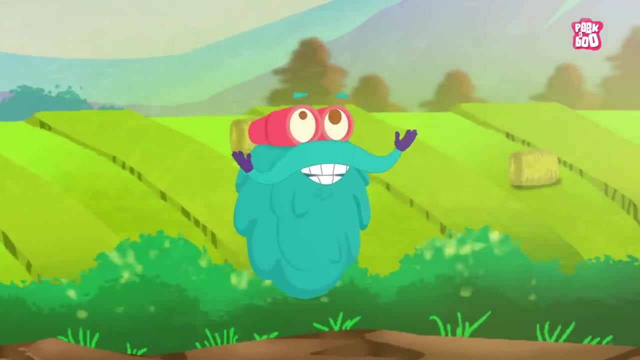 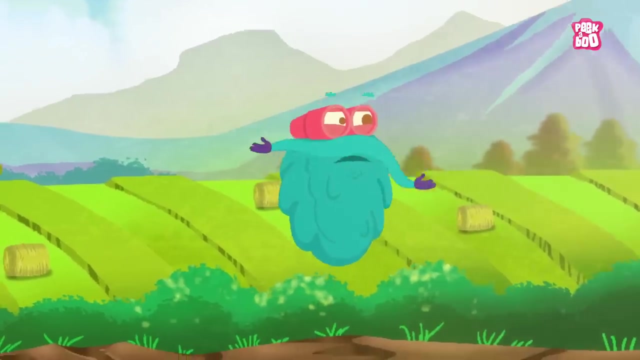 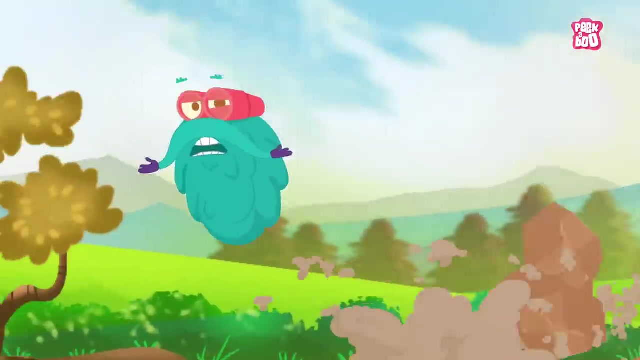 This is me zooming out. Tune in next time for more fun facts. Hey friends, Isn't the weather lovely? Wait a minute, Is it me or is the ground moving? Whoa, Be careful, It's a landslide. Let me tell you about this natural disaster. 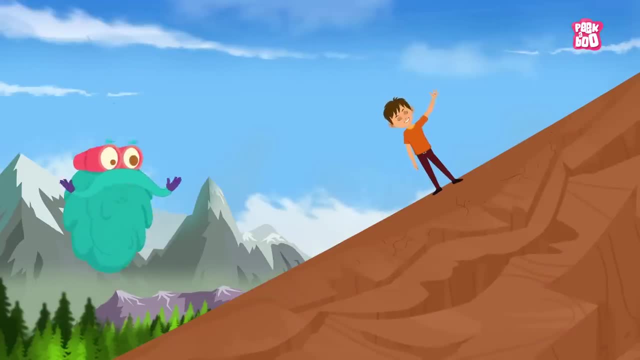 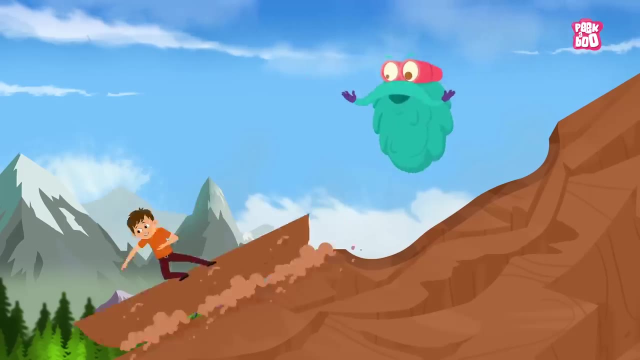 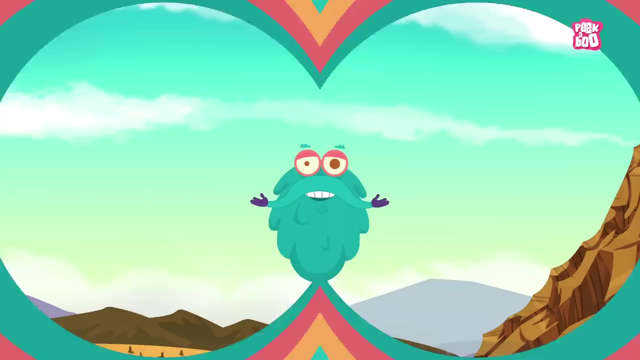 Zoom in. When the upper mass of the soil gets dislocated from the lower layers and travels down slope, it is referred to as a landslide. It is also called a landslip or a mudslide. Landslides can be caused by a number of reasons. 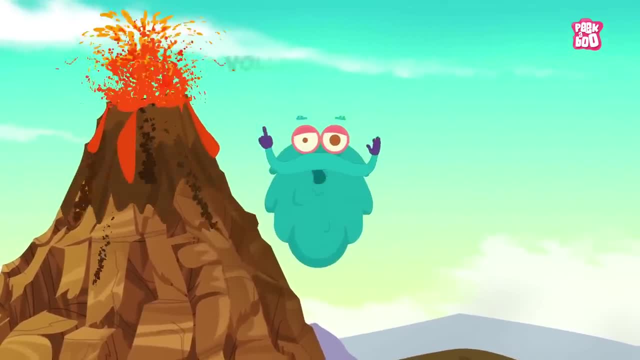 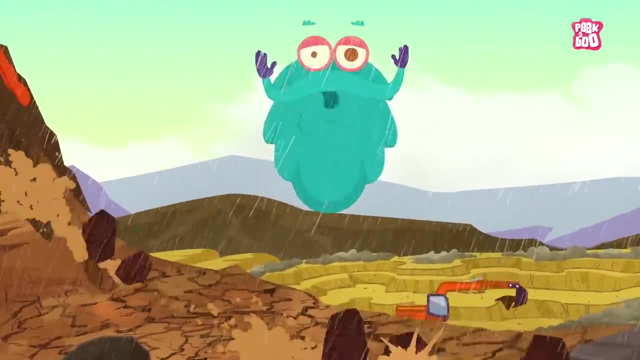 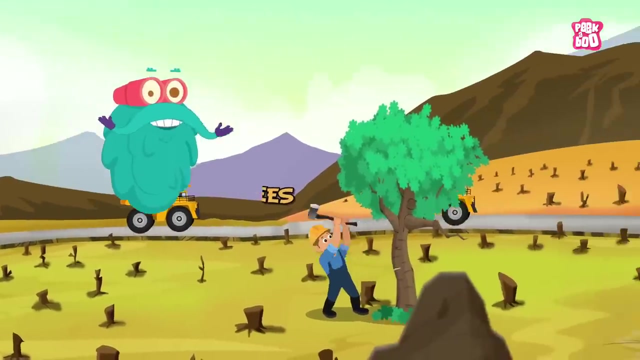 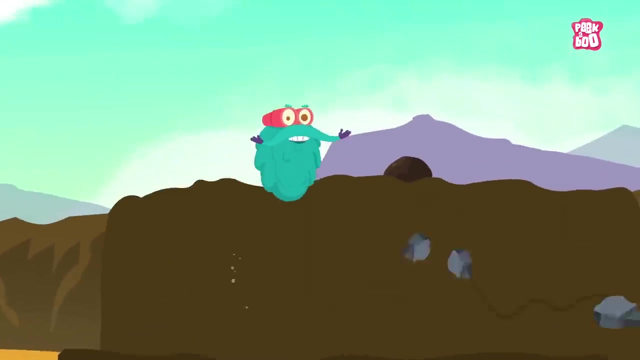 It could be either natural causes like volcanic eruptions, soil erosion and sometimes heavy rainfall. It increases the wrath of landslides. Even human activities like mining, cutting trees, increase the fertility of land and make it more prone to landslides. One of the most prevalent reasons is gravity. 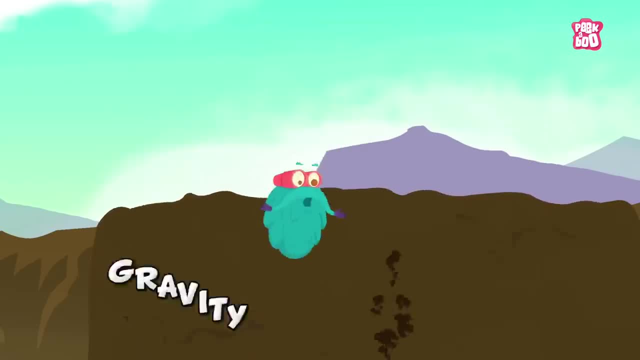 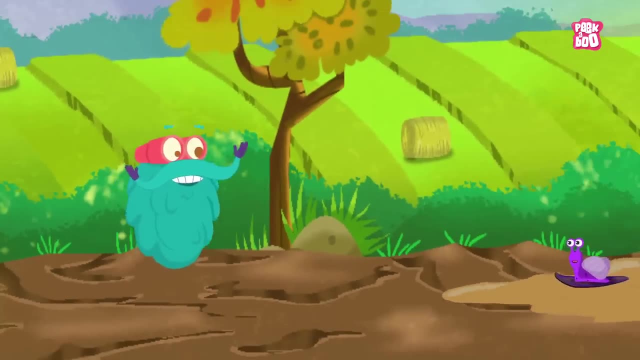 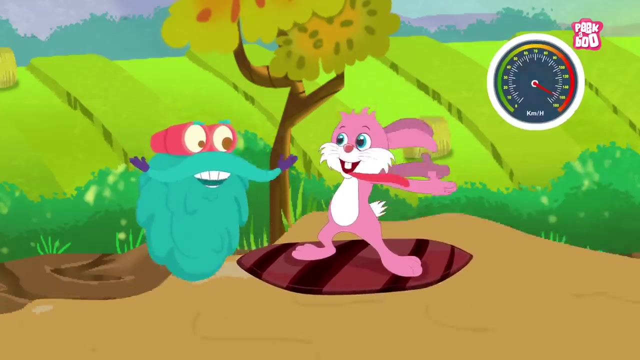 Well, whatever is up has to fall down due to gravity, isn't it? Landslides can either move very slowly, like some millimetres per year, or it could be disastrously fast, sometimes more than 100 miles per hour. 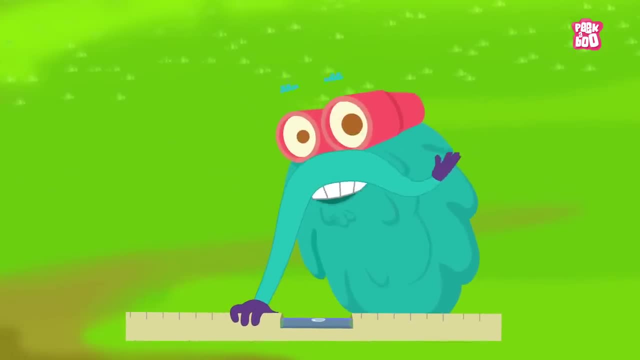 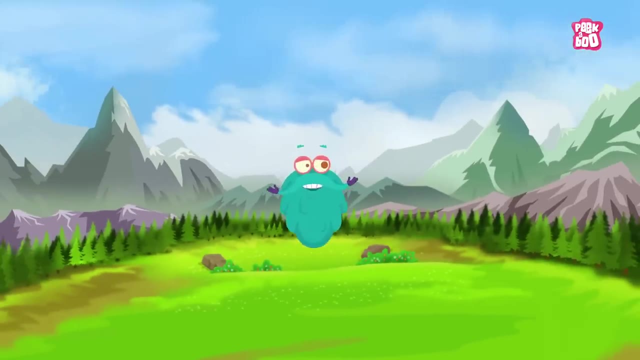 But if you are living on a flat land with no hills or mountains, then you are safe. But if you are living somewhere between mountains and on a hilly terrain, then, my friends, you might be at risk. But don't worry, You could always prepare with some simple steps. 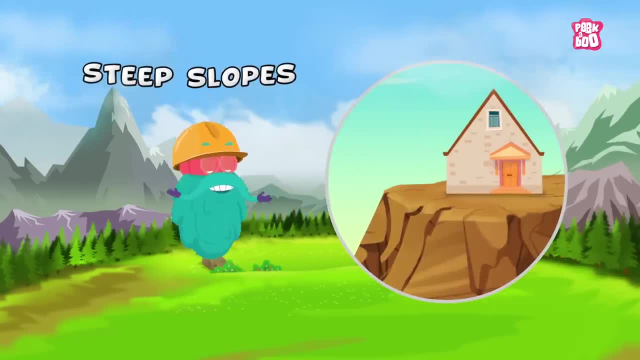 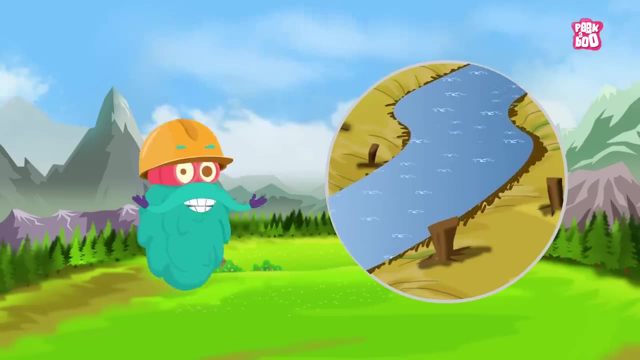 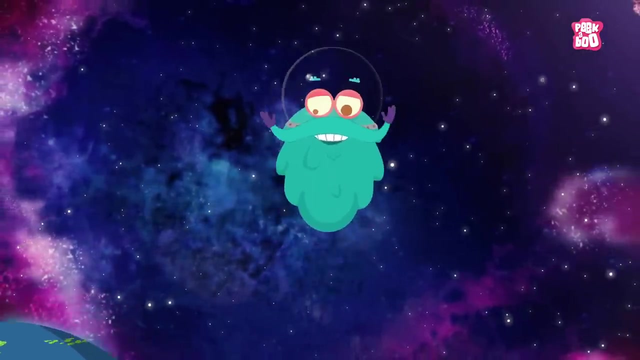 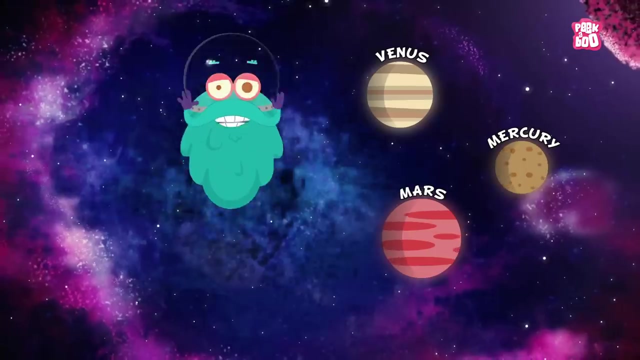 Avoid building houses near steep slopes or at the edges of mountains. Stay away from drainage paths, because water flow increases the speed of landslides. Landslides do not only happen on earth. Many scientists believe that planets like Mercury, Mars and Venus have had landslides too. 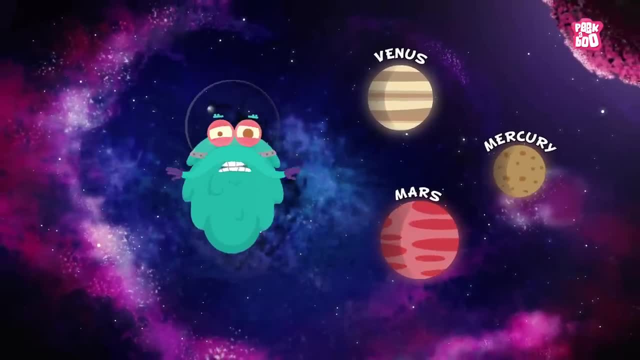 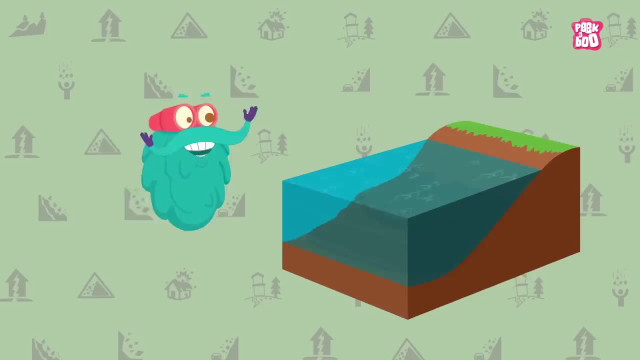 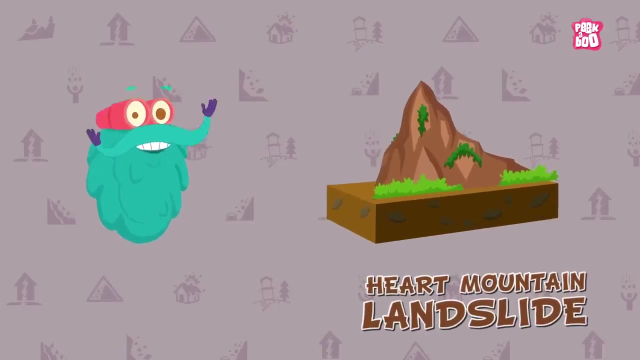 Whoa Looks like friends. I am not even safe here. Trivia time. Landslides can happen underwater too, and they are called Submarine Landslides. The Heart Mountain Landslide is the largest landslide ever recorded. that has happened 50 million years ago. 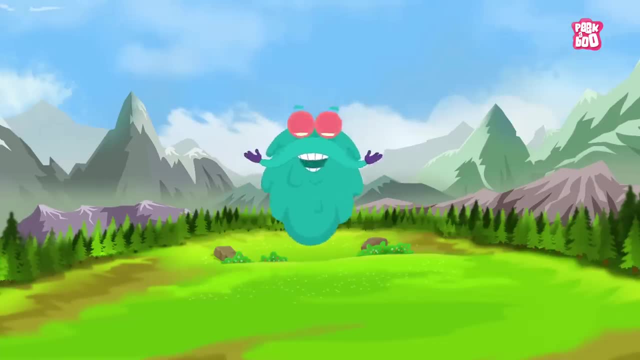 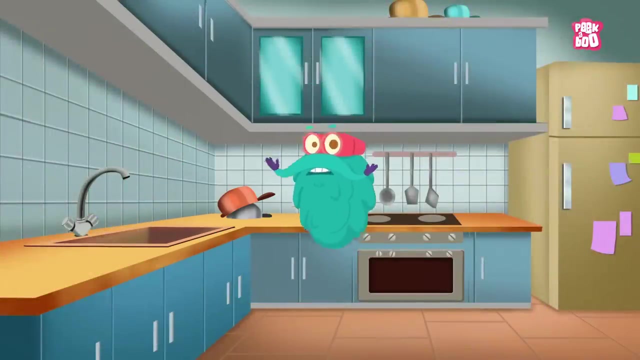 So, friends, what are the other two names for landslides? Post it right below in the comment section and wait for more fun facts. This is me zooming out. What's wrong with the water today? One day of no water can be so troublesome, isn't it? 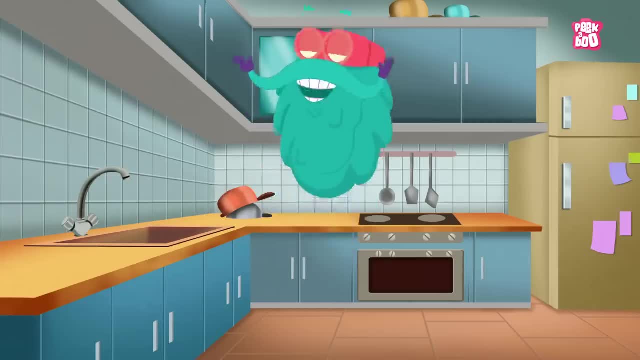 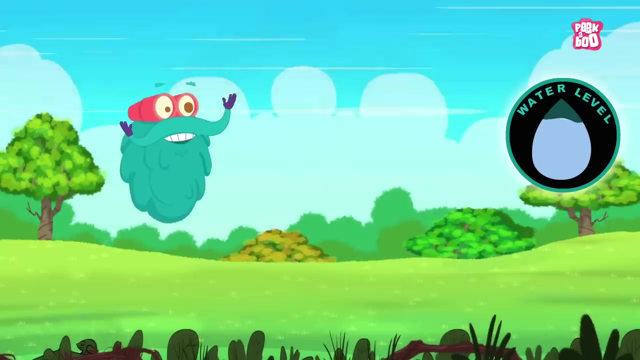 But can you imagine living for a week without adequate water supply? That's what happens in a drought, And this is what we will be talking about today. Come on, zoom in. Droughts are usually defined as extended periods of time with less than average rainfall. 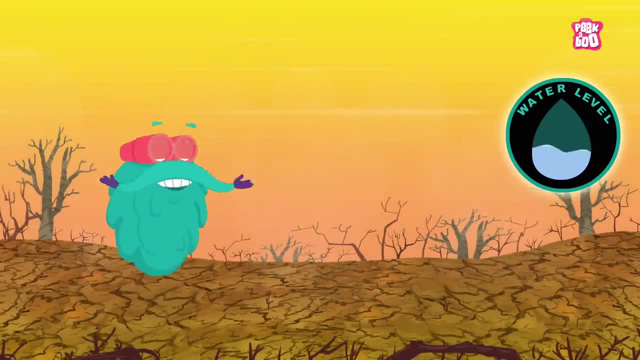 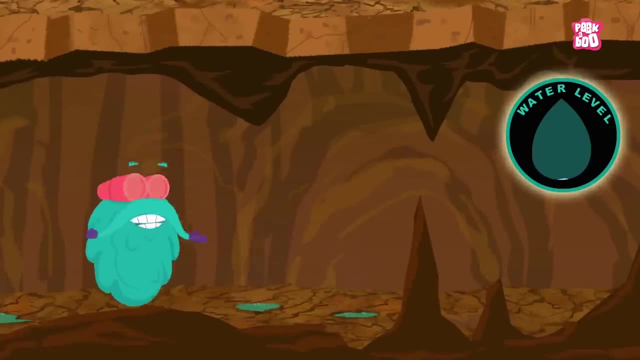 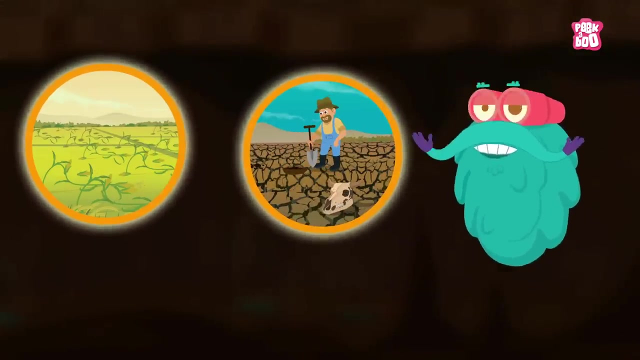 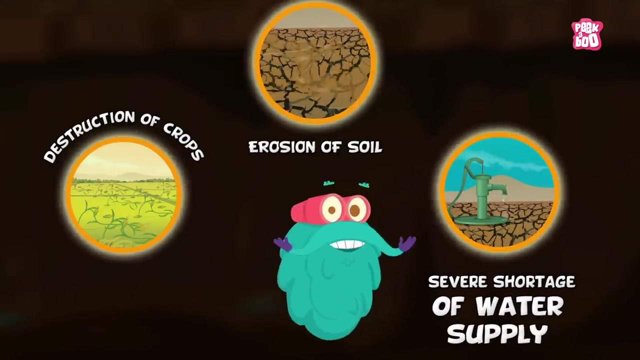 Causing a water shortage on the surface, in the atmosphere or in the ground water levels. It truly becomes a disaster when it begins to affect crops and the lives of people and animals alike. Droughts can lead to the destruction of crops, erosion of soil, severe shortage of water supply, etc. 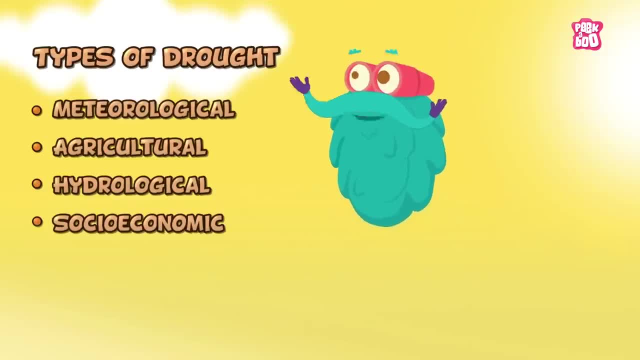 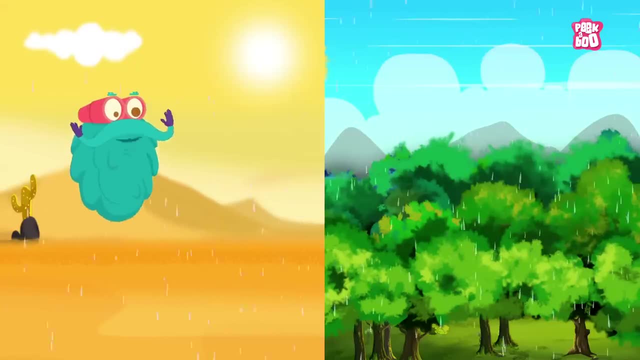 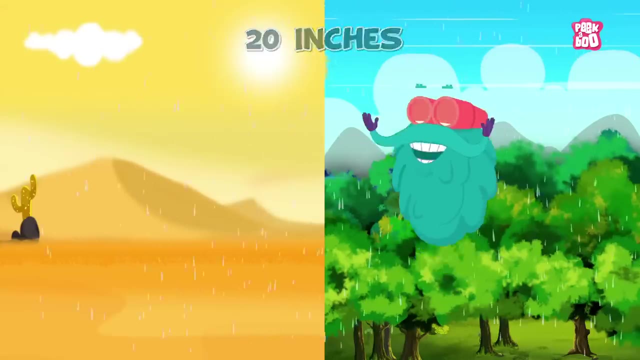 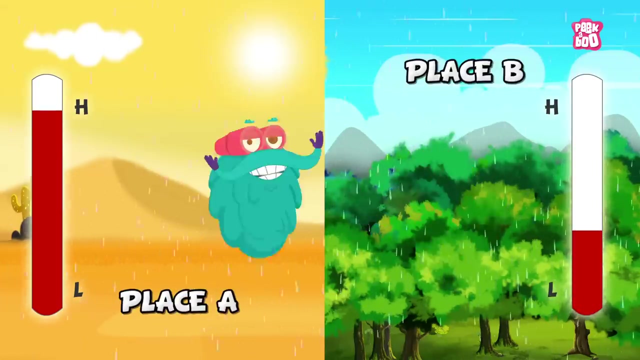 Droughts can be classified into four different types. These are: Meteorological Drought. This kind of drought is specific to different regions based on the weather. For example, 20 inches of rainfall in a year is normal for place A, But the same amount could be very less to place B. 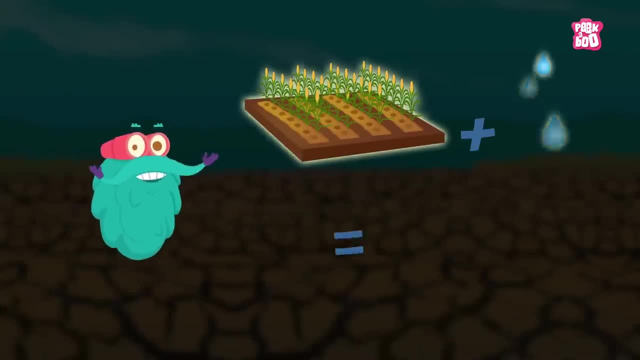 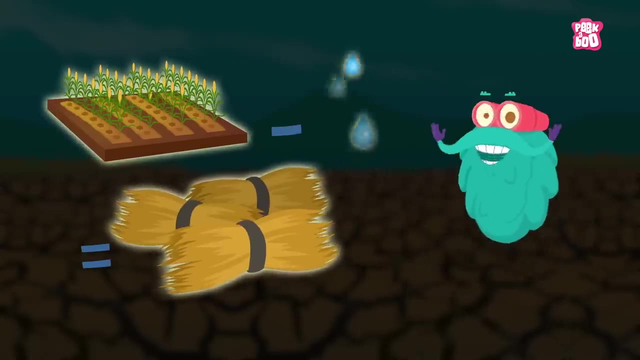 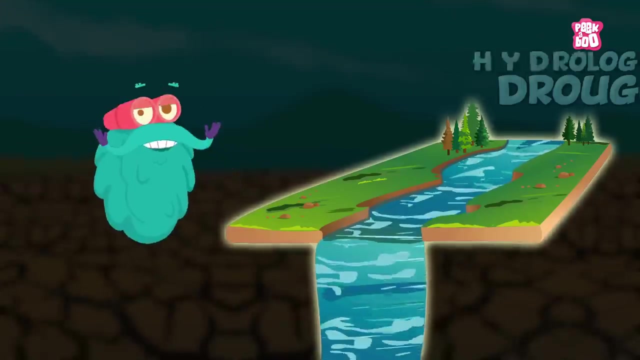 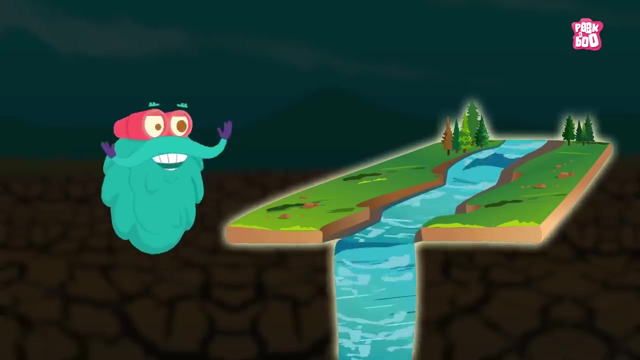 Agricultural Drought. This accounts for the water needs of crops and agriculture, For instance. not enough water at planting may cause low yields, Leading to low plant populations. Hydrological Drought refers to continuous low water volumes in streams, rivers and reservoirs. 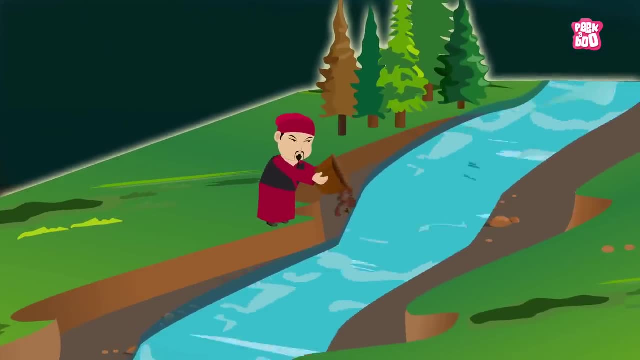 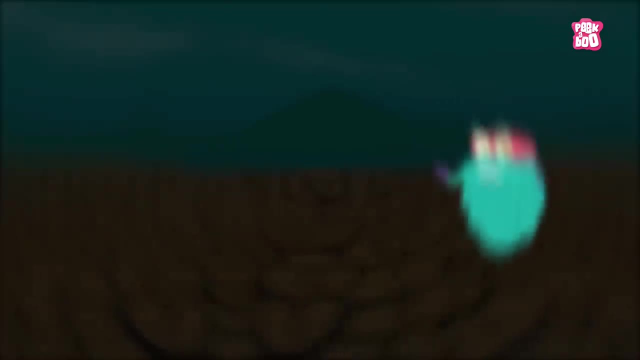 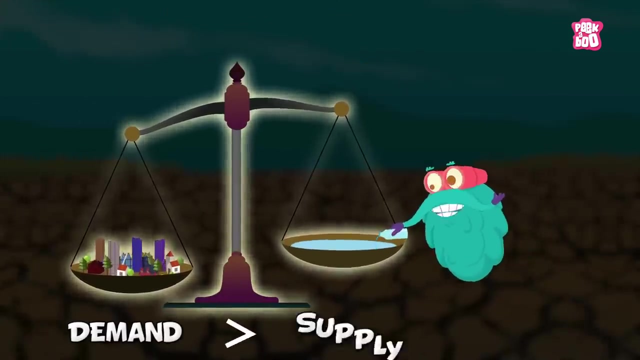 Human activities can worsen hydrological droughts. Hydrological Drought is often linked with Meteorological Drought- Socioeconomic Drought. This occurs when the demand for water exceeds the supply. Examples of this could be When a state requires a lot more water. 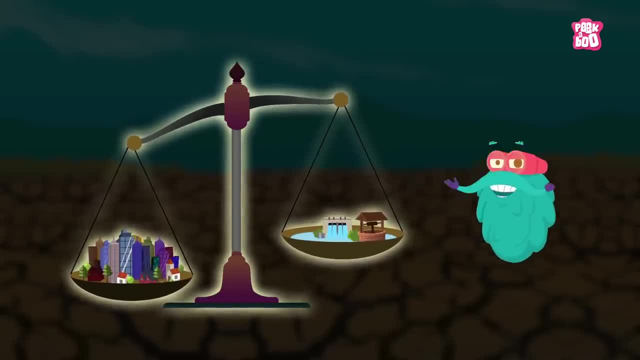 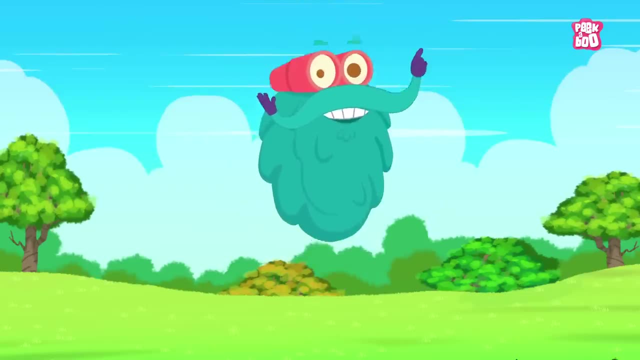 More water than is produced from hydroelectric stations or underground wells. Now that you know about what droughts are, Let me tell you some tips on how to survive them. The one major rule you must keep in mind is Save Water. So here are some tips for saving water during a drought. 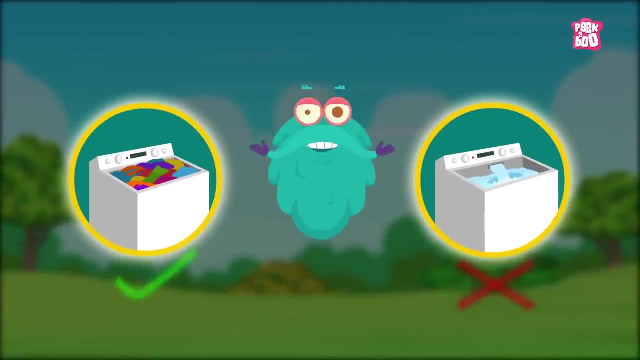 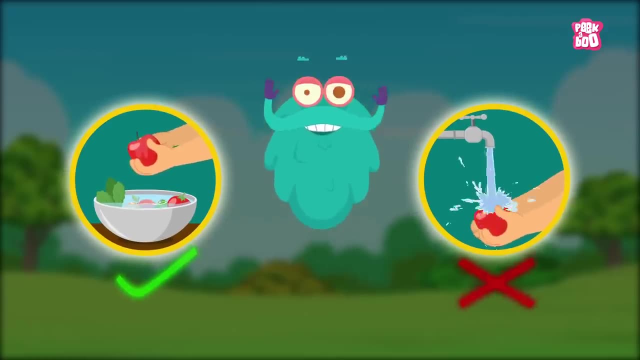 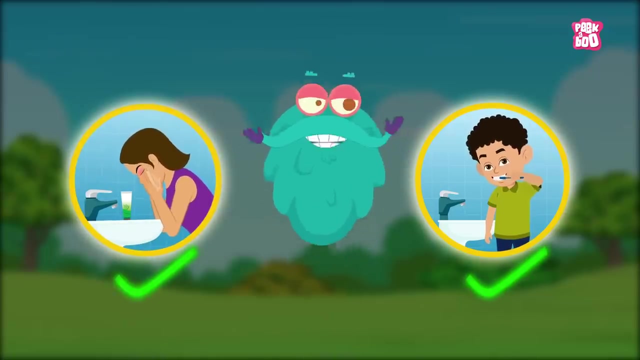 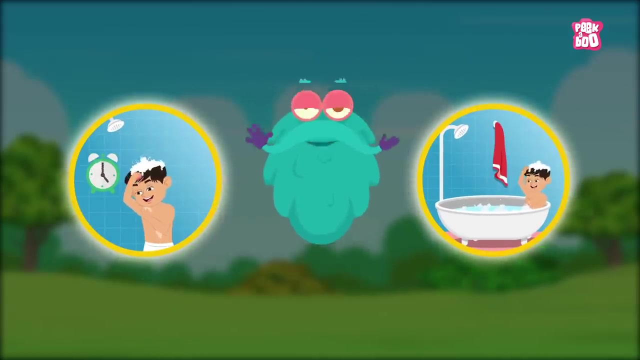 Fill the washing machine and dishwasher to full before starting them. Wash fruits and vegetables in a bowl of water instead of under running water. Don't leave the water running while washing your face or brushing your teeth. Take smaller showers or, if you use a bathtub, fill it only half way. 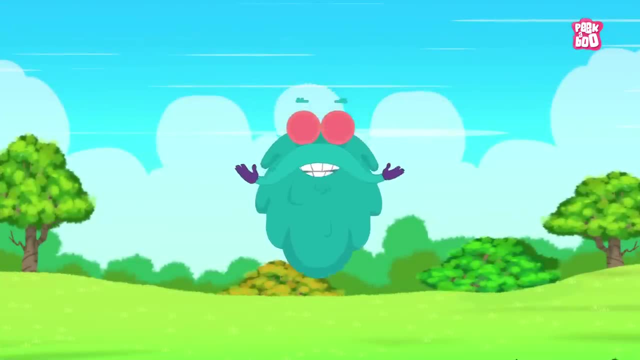 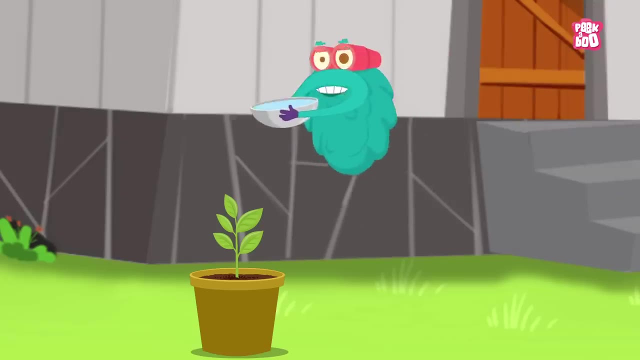 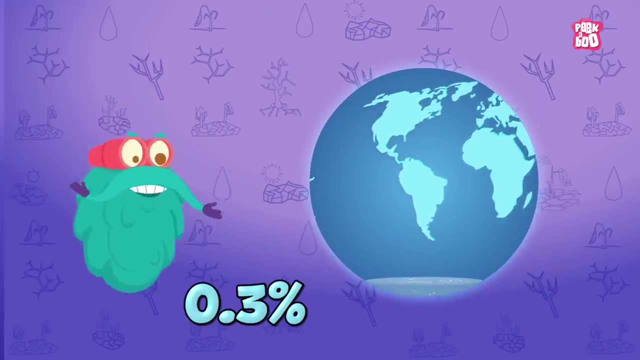 And, most importantly, recycle. Don't waste water that can be recycled. Reuse it somewhere else, Such as to water plants or cleaning Trivia Time. Only 0.3% of water on earth is fresh water Available for human consumption. 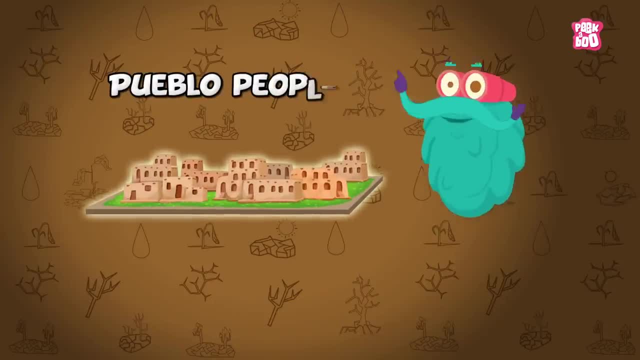 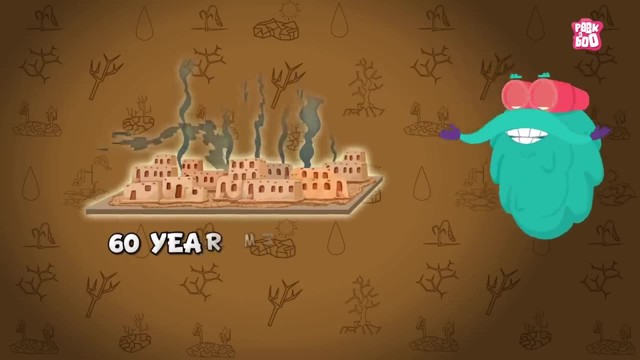 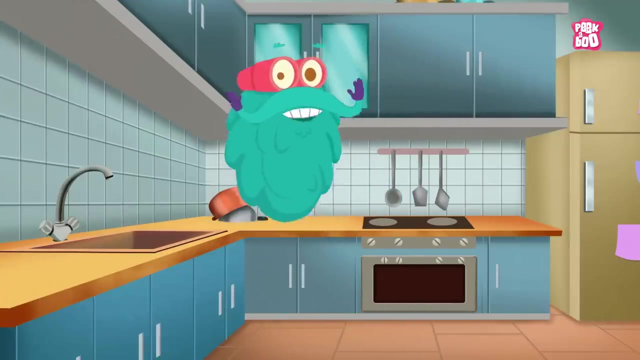 A once thriving settlement by the Pueblo people in Chaco Canyon, New Mexico, was abandoned in the 13th century due to a 60 year mega drought. Well, friends, now you know what droughts are and how to prepare and survive through them. 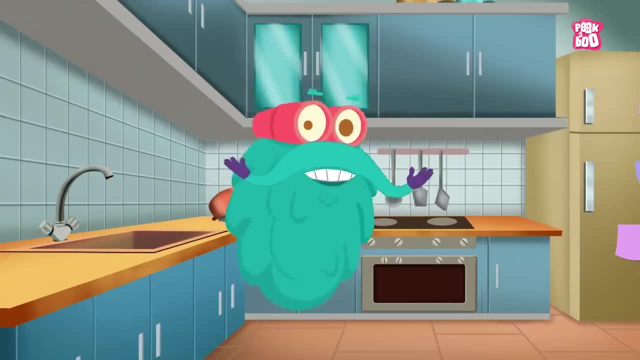 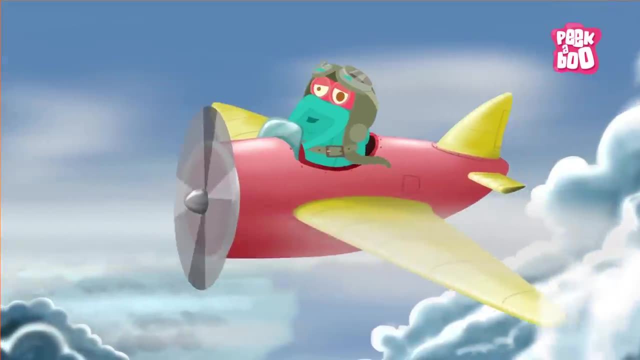 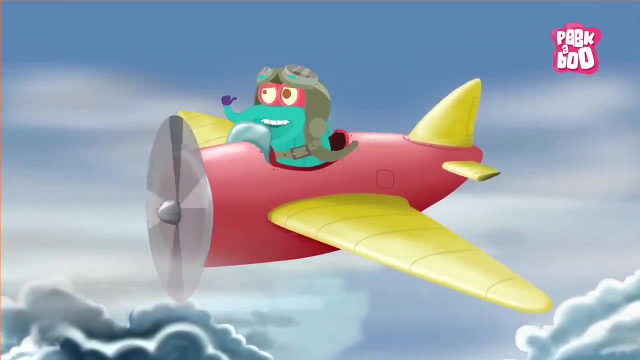 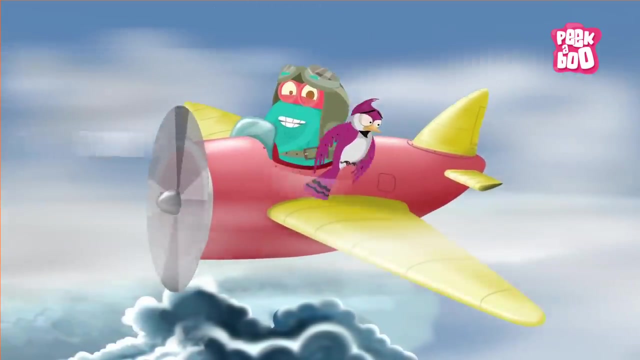 For more fun facts, tune in next time. Till then, this is me zooming out. Hello, It's quite windy today, so I thought I'll take a quick flight. Oooh, It sure is windy. Oh no, It's a storm. 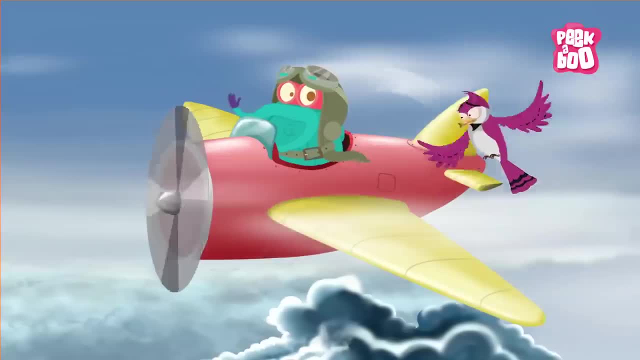 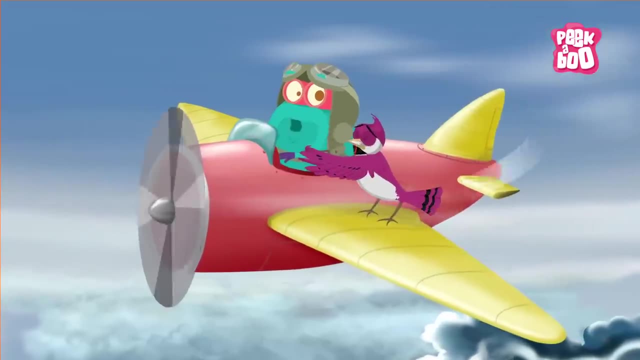 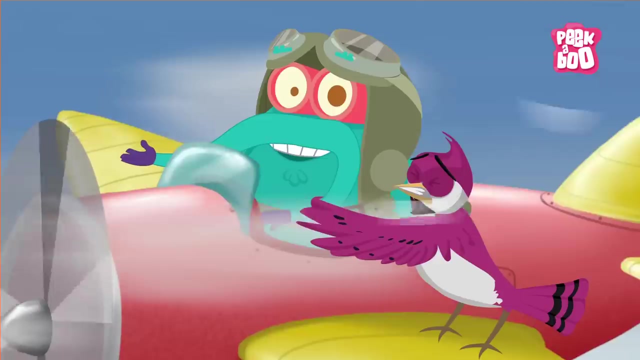 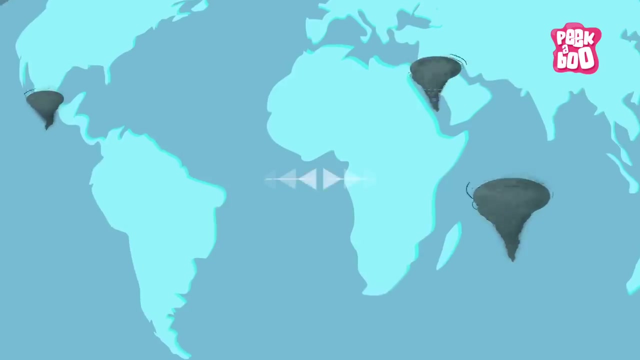 You mean hurricane, Hurricane Storm, Whatever? Just run. You mean fly? Oh, forget it. Just come, Dr Binocs. Oh, okay. Well, that reminds me that today's topic is hurricane Zoom in Whoa. A hurricane is a huge storm that generally forms over warm ocean waters near the equator. 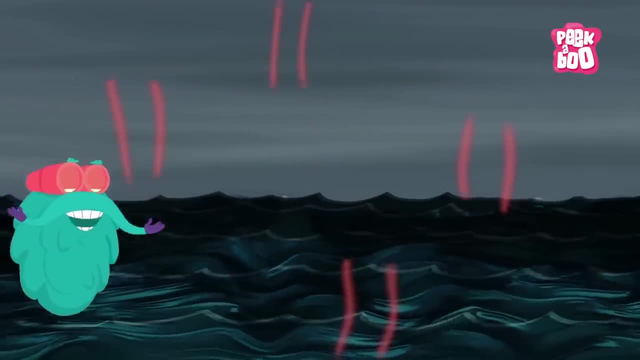 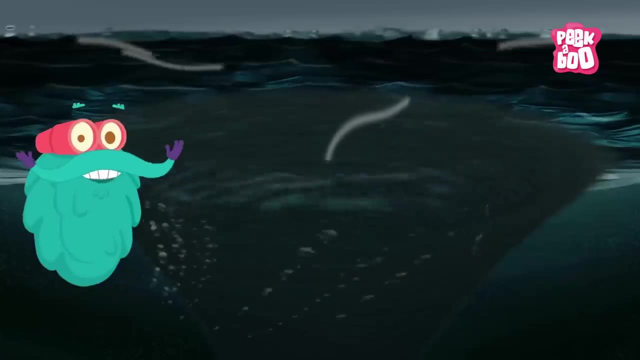 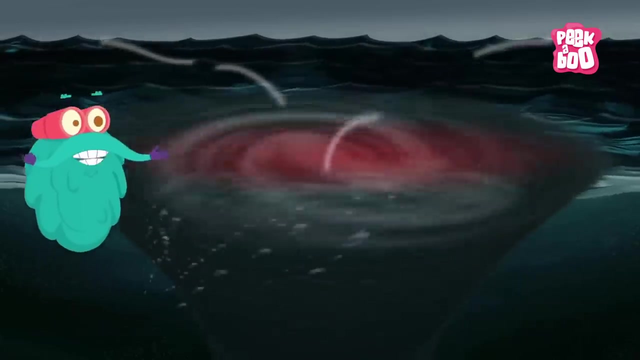 The warm air above the ocean rises upward, thus creating an area of low pressure below Air from the surrounding areas. push in and try to fill the area with low air pressure, which now becomes warm and moist and rises too As the moist air rises. 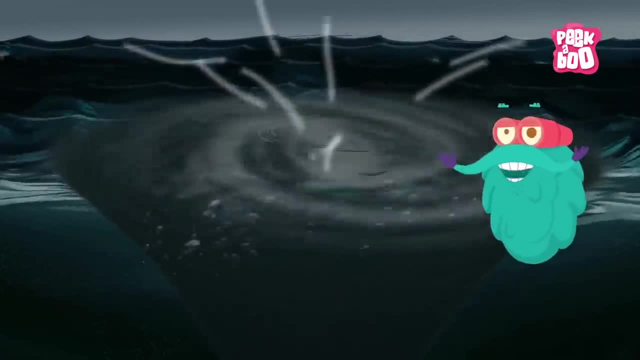 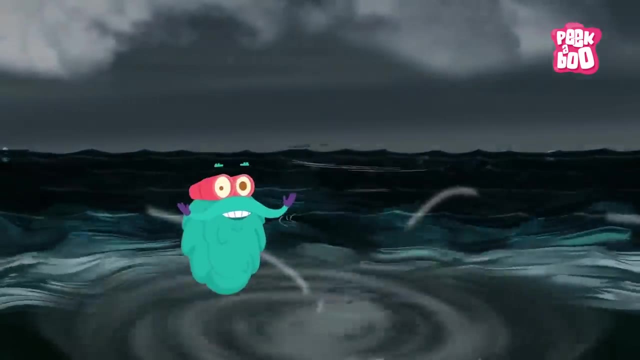 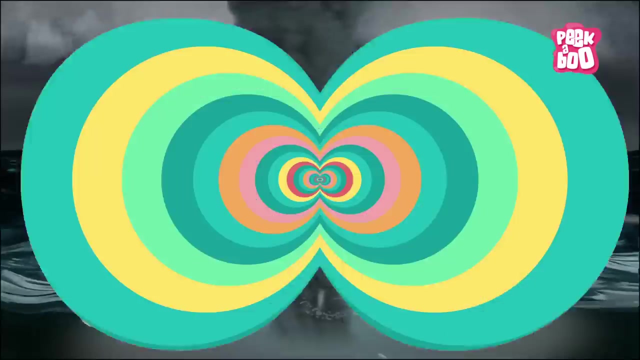 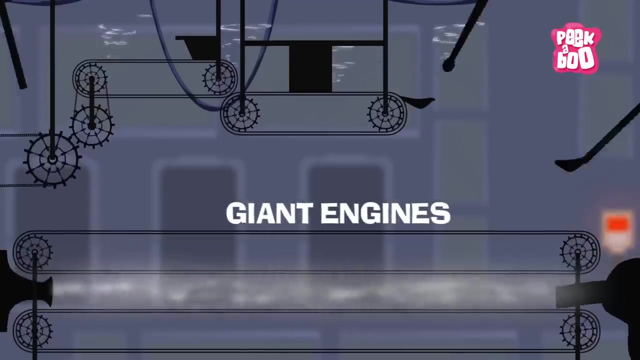 the surrounding air again tries to fill in, And this process continues till the water in the air forms clouds. Soon, the clouds and winds spin around, fueled by the ocean's heat and water vapor. Therefore, hurricanes could also be called giant engines that use warm and moist air as their fuel. 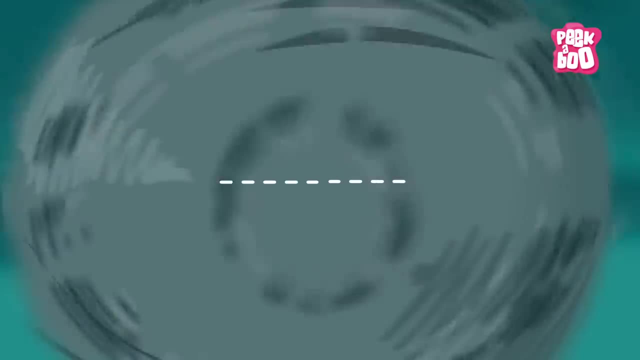 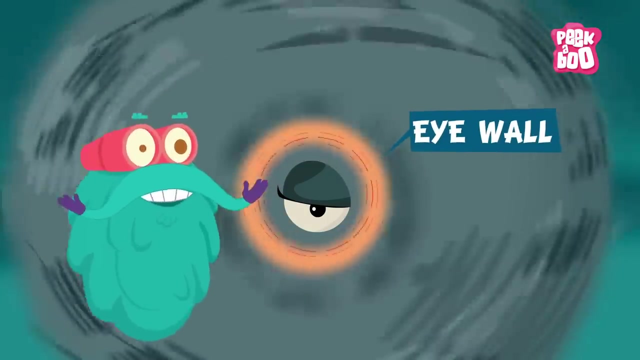 When we see from the top, hurricanes can be as huge as 300 miles wide. The center of the hurricane is called the eye of the hurricane, which is the calmest part. The eye wall surrounds the eye, where the most damaging winds are found. It can range anywhere from 5 to 30 miles. Then comes the rain bands which surround the eye wall. These bands are a series of dense clouds that give a pinwheel-like appearance to the hurricane, which range from 50 to 300 miles. Hurricanes are divided into 5 categories depending on the speed of their wind. Here take a look. Category 3, 4 and 5 are the most dangerous ones. Trivia time: A huge hurricane can release energy equivalent to 10 atomic bombs per second. 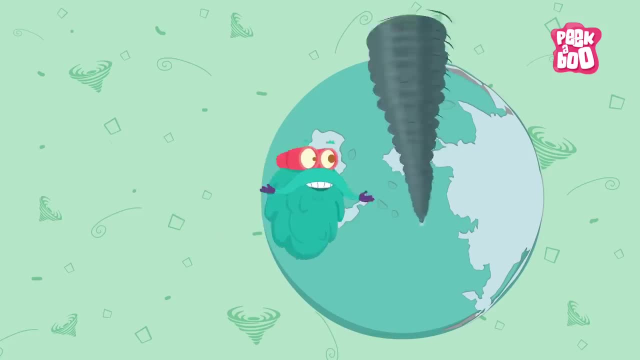 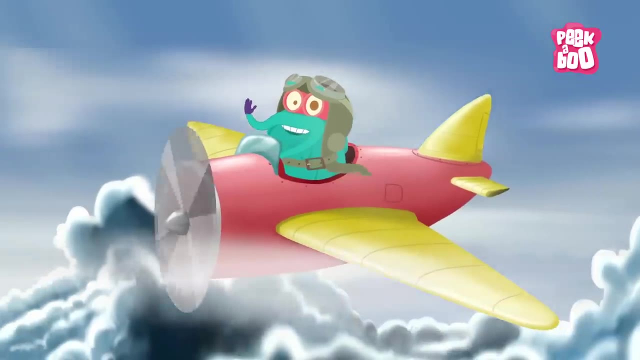 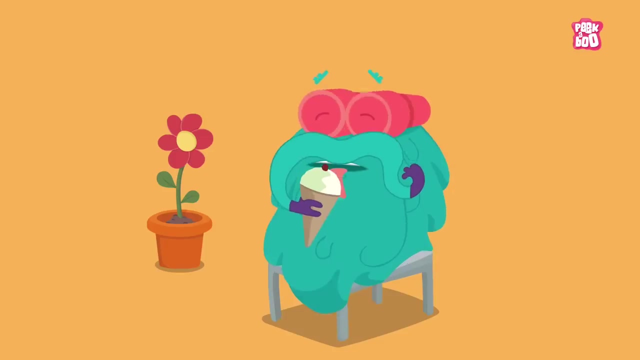 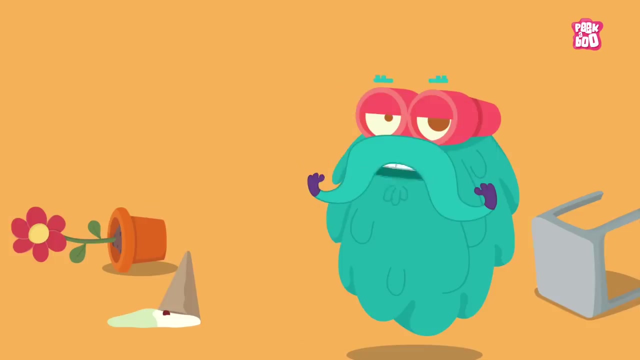 Hurricanes in the Pacific Ocean are known as typhoons Whoa. So this is me zooming out. Tune in next time for more fun facts. Bye, Whoa. You're laughing right Watching me tumble like that, Are you? 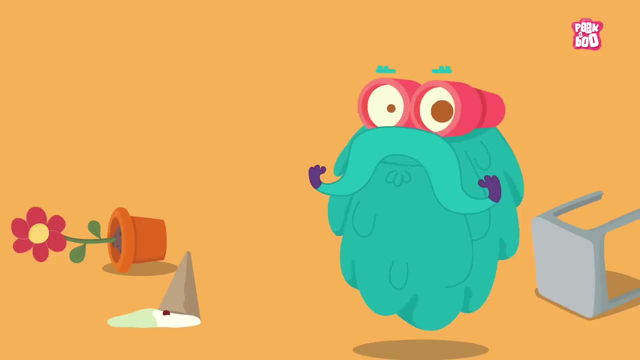 Oh, No, no, Go ahead. But hey, Do you know what just happened? There we go again. Well, this is nothing but an earthquake, A small one indeed. Come, let me tell you about earthquakes today. Zoom in. 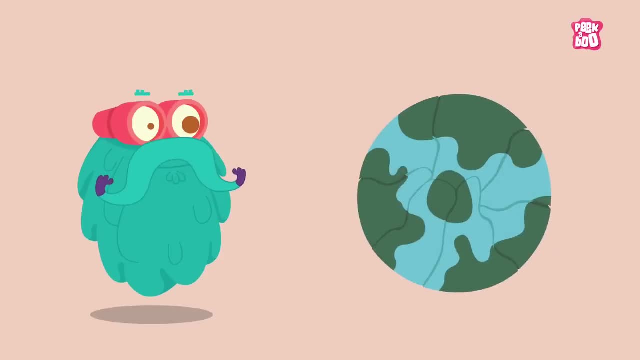 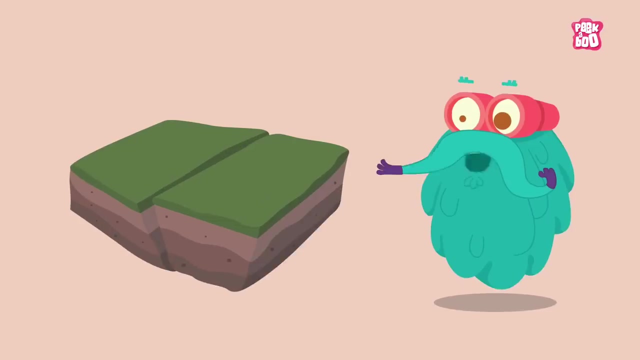 The surface of the earth is like a jigsaw puzzle. Yes, it's not a single piece of land, but approximately 20 pieces of a puzzle that constantly move. But you don't feel it because they move quite slowly. Each one of those puzzle pieces are called tectonic plates. 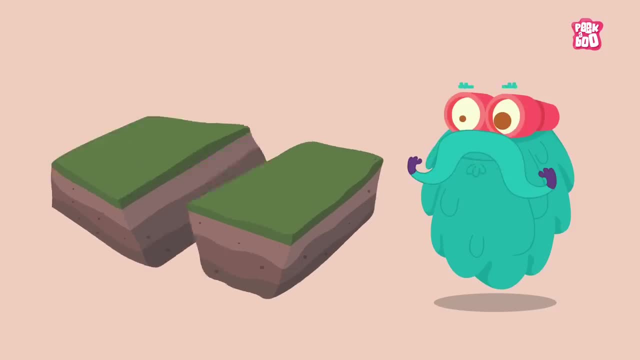 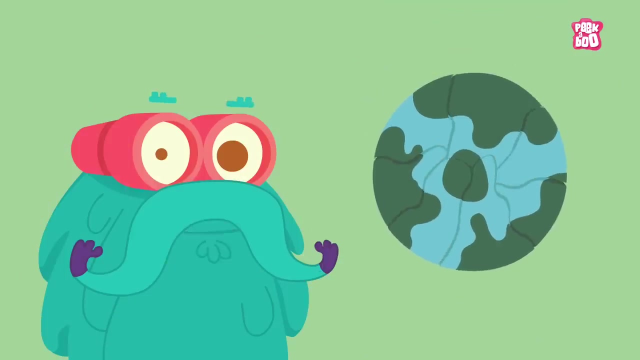 So whenever those plates hit, bump or slide past another plate, an earthquake is caused. The surface where these plates slip is called the fault or the fault plane. So when do you think it happens? Well, it happens all the time. 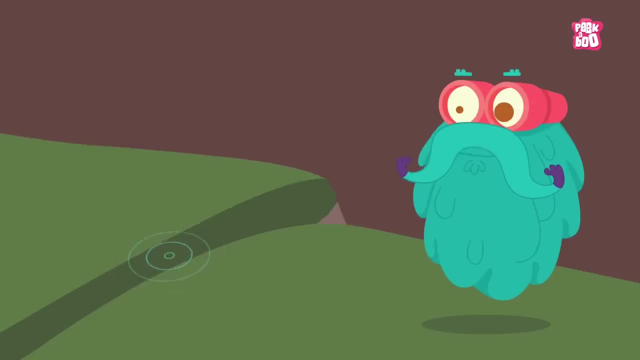 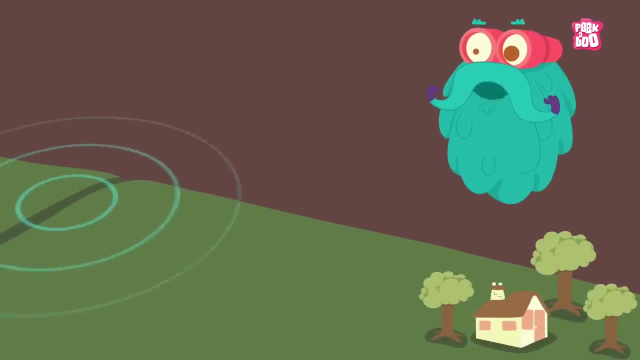 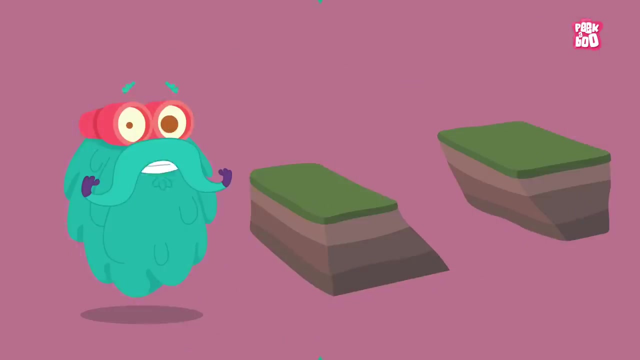 But hey, Don't be scared. Most of the times we don't feel the quakes As they are too small to reach us, But sometimes they are so strong that they can be felt over a thousand miles away. The place where the earthquake originates is called the hypocenter. 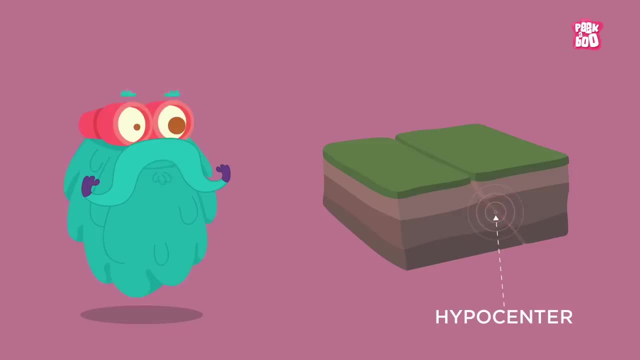 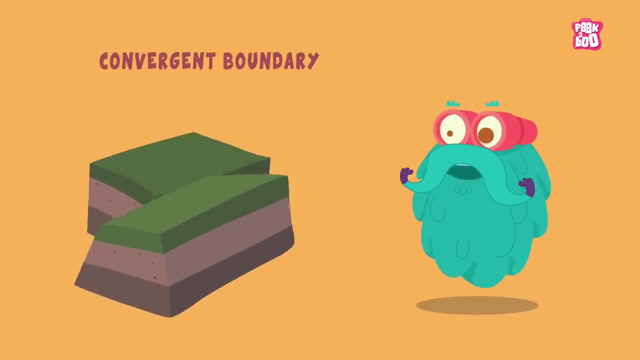 And the place where it occurs on the earth's surface is called the epicenter. There are three types of earthquakes: Convergent boundary: Here one plate is forced over another during an earthquake, which causes a thrust fault. Many hills and mountains have been formed due to the convergent boundary. 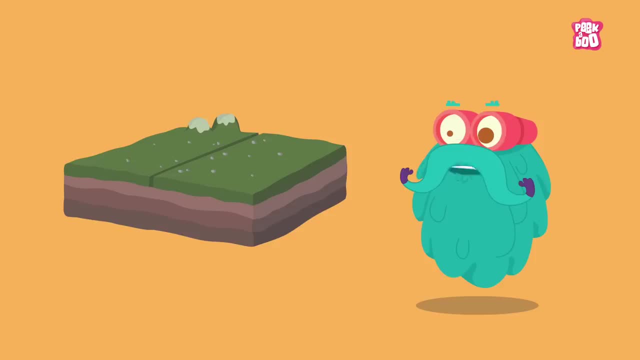 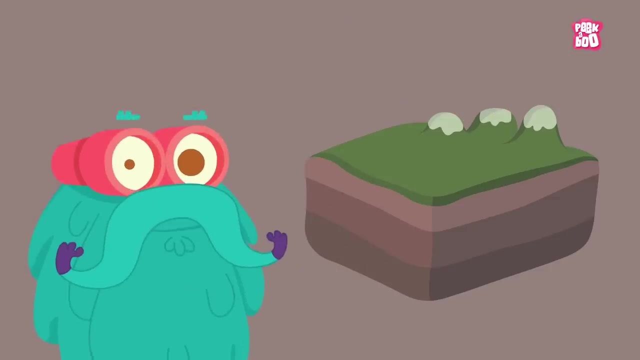 Divergent boundary: Here plates are drifted apart from each other, forming a rift zone. This kind gives birth to new ocean flows. Transform fault: Here the plates slip by each other And this is also called strike-slip. So earthquakes are nothing but the shaking, rolling or a sudden shock of the earth's surface. 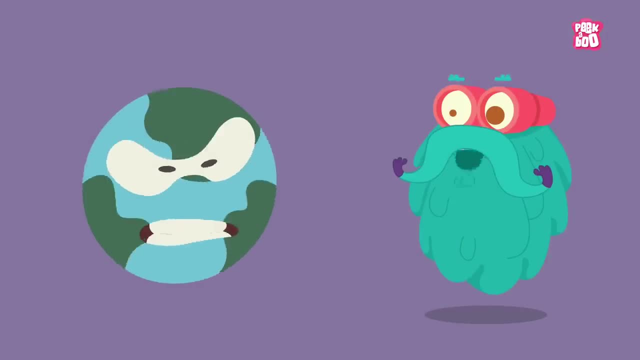 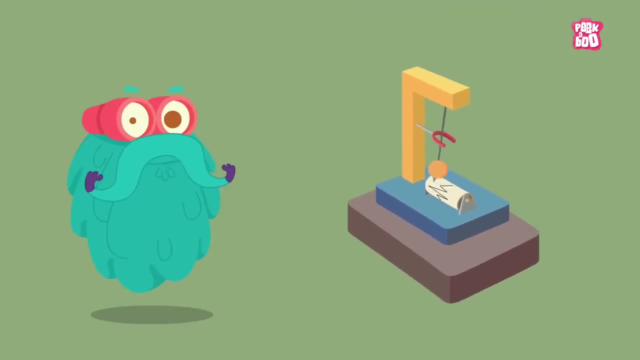 Now you know that whenever the earth is stressed or angry, it shakes and grumbles. Don't be scared, I was just kidding, Trivia time. The instrument used by scientists to measure the intensity of earthquake is known as a seismograph. 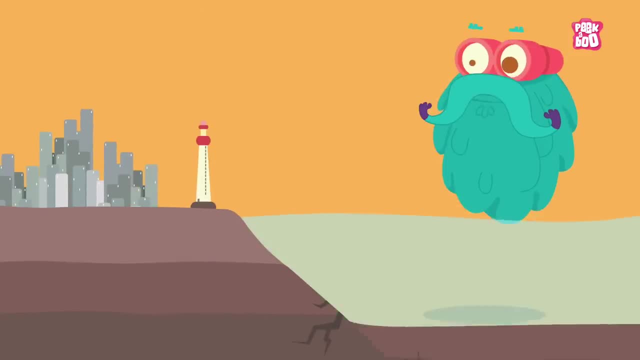 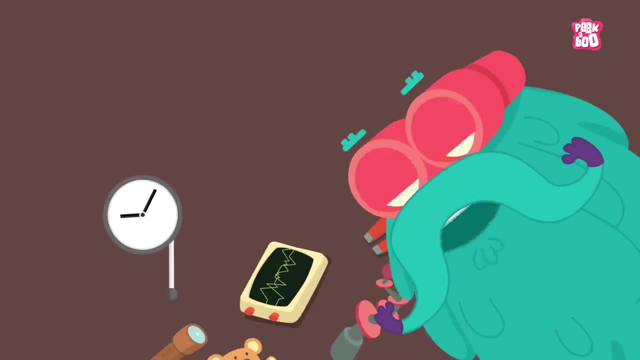 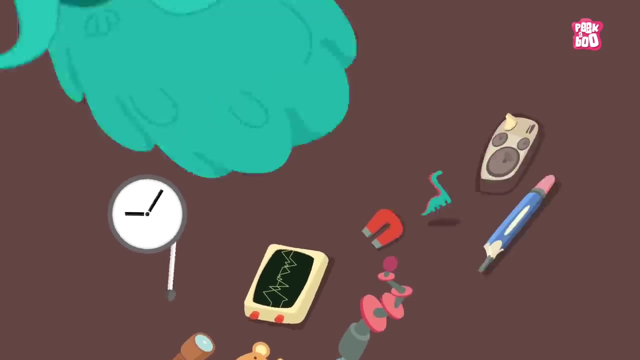 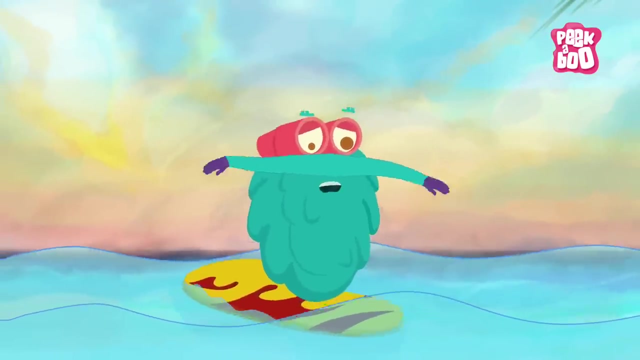 A tsunami is caused when earthquakes occur under water. Whoa, Yikes, I need to rush before I tumble again. So this is me zooming out. Tune in next time for more fun facts. Hey, Hello friends, Oh no. 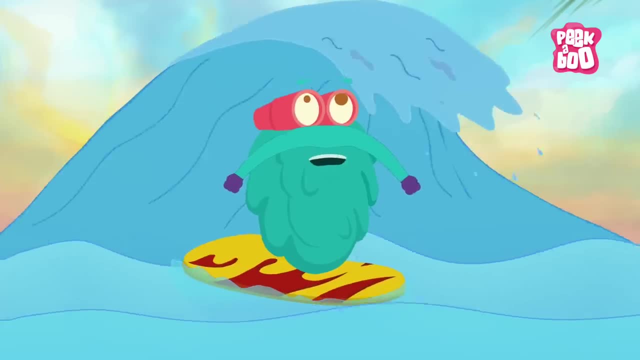 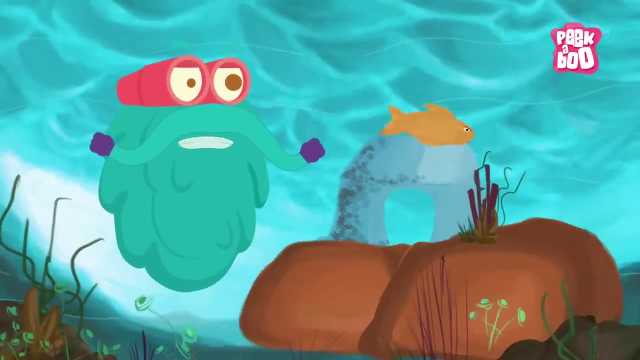 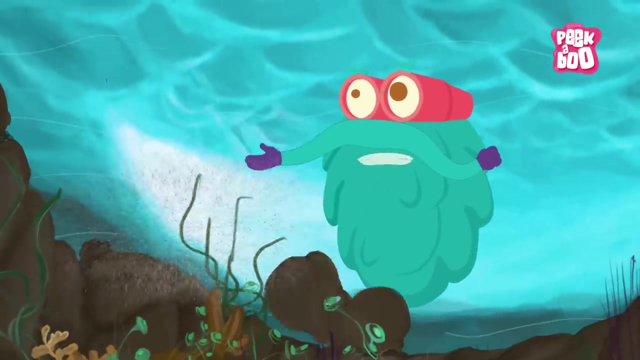 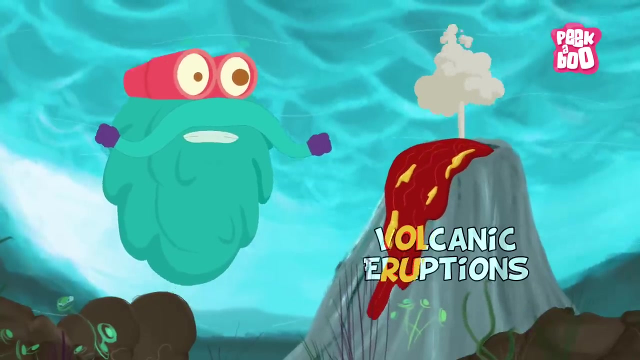 I guess that's a tsunami. Come. Let me tell you all about it. Zoom in. Tsunamis are caused by the sudden movements of the ocean floor due to earthquakes, Landslides on the sea floor, land slumping into the ocean, large volcanic eruptions or a meteorite crash on the ocean floor. 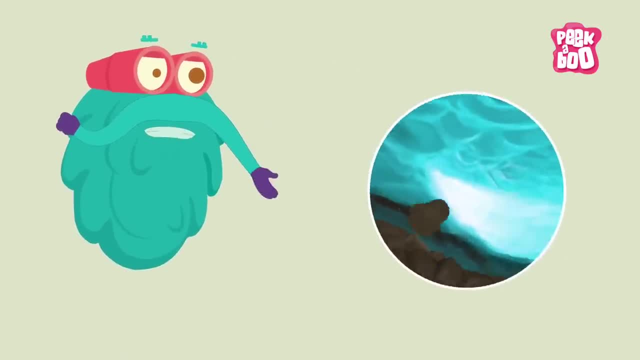 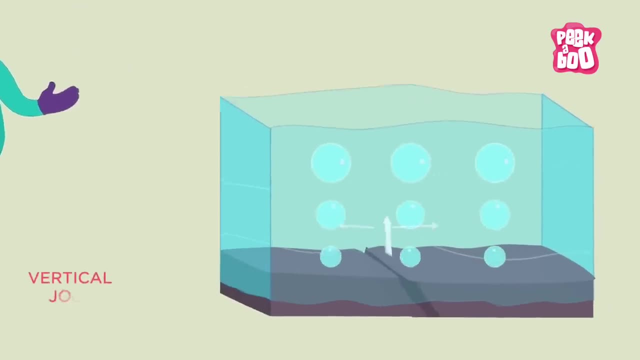 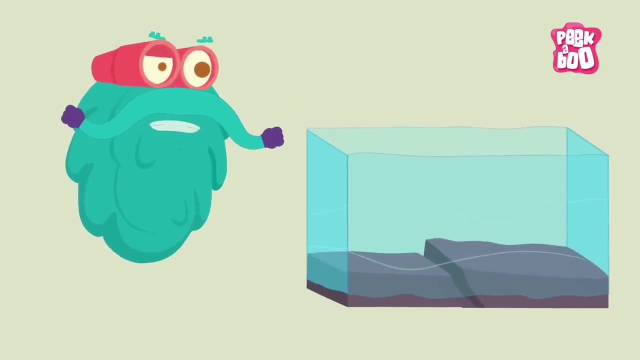 When an earthquake, a landslide or a volcanic eruption occurs on the sea or ocean bed, a vertical jolt is created which displaces the bed and causes extreme tension in water. The water is pushed upwards, but gravity tries to pull it down. This causes an upsurge in the water levels and the waves start moving away from the point of tension. Tsunamis are barely felt as a ripple on the ocean surface, as the water is quite deep. But as and when those waves reach the land, the water becomes shallower And the waves constantly increase in height. They hit the shore and, oh my, cause a lot of destruction. 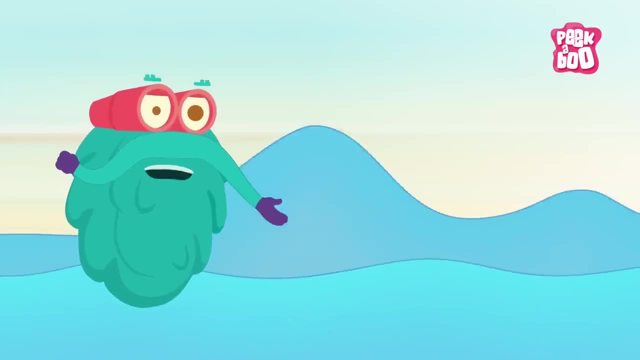 It is said the first wave of a tsunami is not the strongest, But the successive waves are bigger and stronger. Oh And, tsunamis can travel at a speed of about 500 miles per hour, Which is almost as fast as a jet plane. 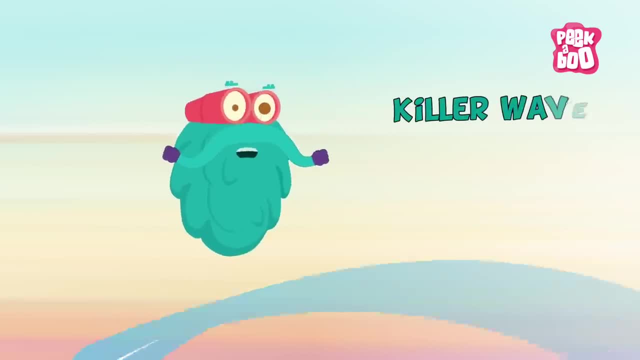 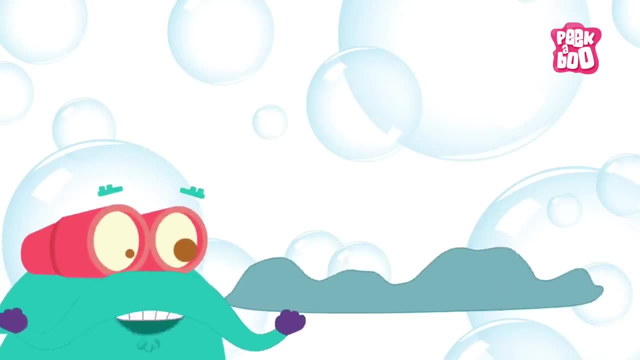 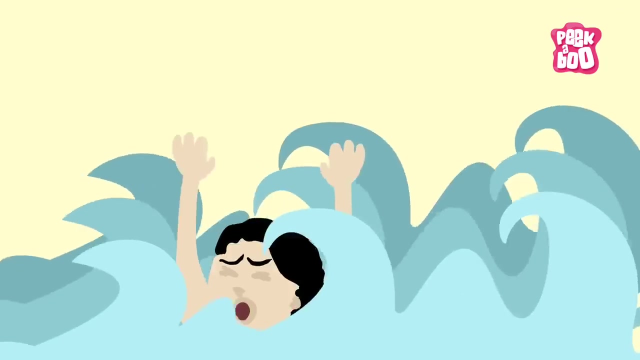 And that's why tsunami waves are called killer waves- Deadly, isn't it? Trivia time? Did you know that a tsunami wave can be less than 30 cm in height and can pass off unnoticed? If you get stuck in a tsunami, don't swim, because the currents will pull you in the opposite direction. 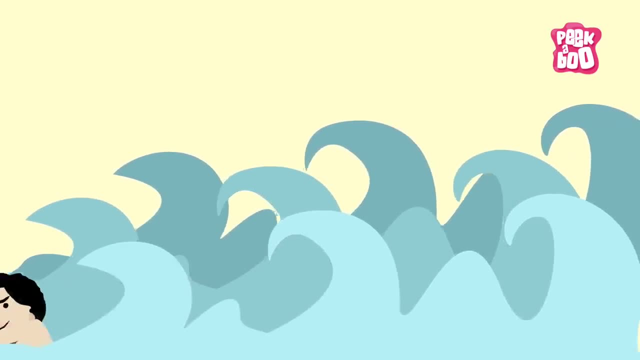 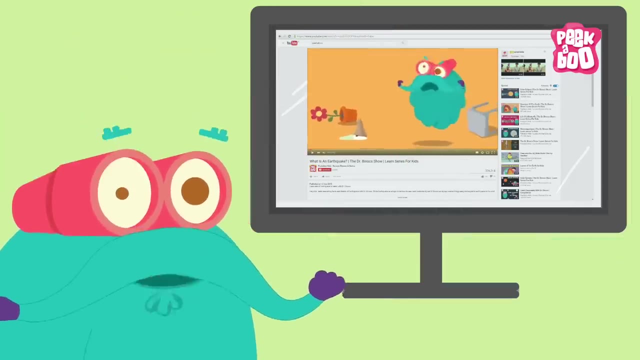 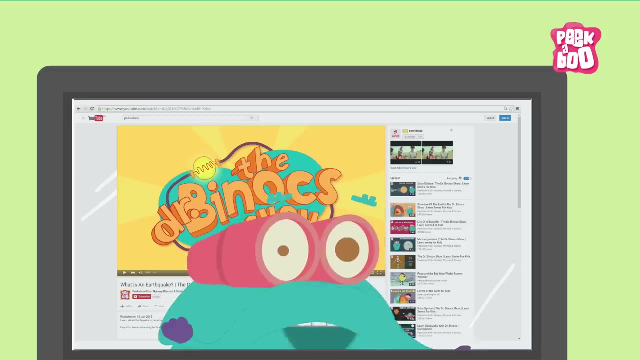 Just hold on to a floating object and be safe. So here's the deal. Go, watch this video to know more about earthquakes. After all, that's one of the major causes of a tsunami. This is me zooming out. Tune in next time for more fun facts. 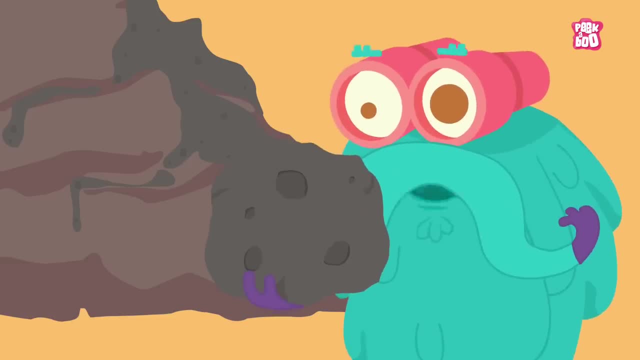 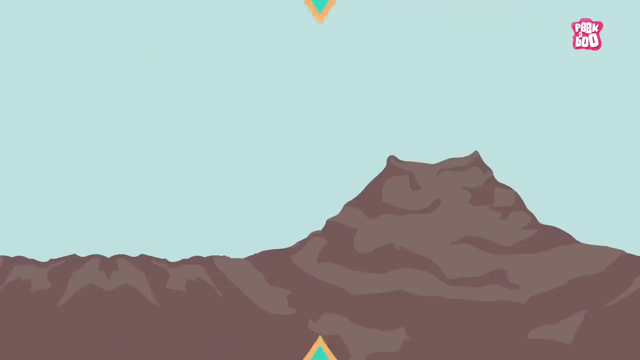 Are you wondering what this is? Well, it's the molten lava that comes out from a volcano. Come, let me tell you what a volcano is. Zoom in. I'm sure you've seen mountains that open up and blurt out thick, molten, semi-solid like substance.